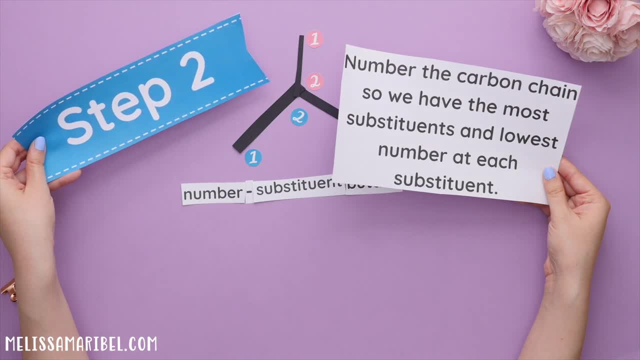 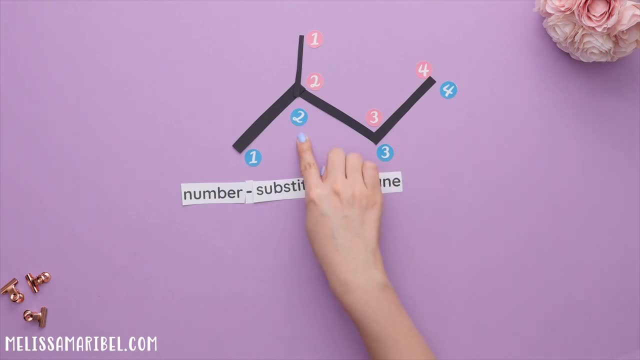 we have the most substituents and the lowest number at each substituent. So if we numbered the carbon chain from left to right, the substituent would be at two. If we numbered it from right to left, the substituent would be at three. So we'll keep it numbered from left to 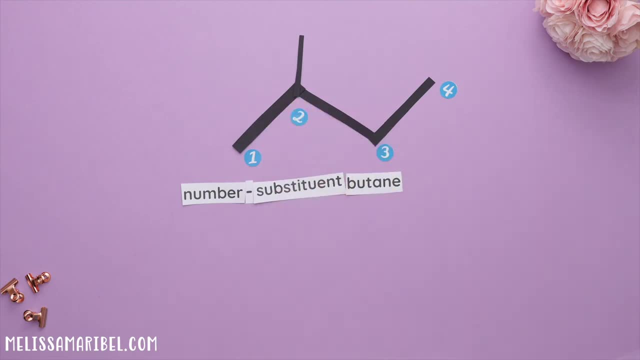 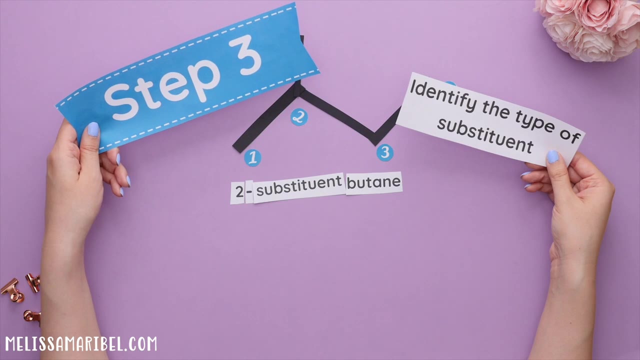 right, since we always want the lowest number for our substituent. Step three: find the longest carbon chain for our substituent. We now know the location of our substituent is at two. Step three: identify the type of substituent. There is only one carbon that is not already part of the main. 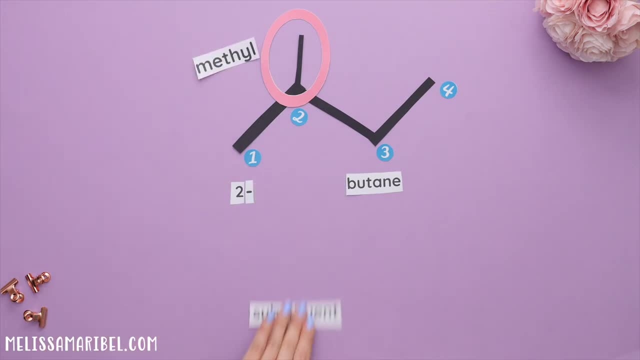 carbon chain. so this is a methyl group and we get two dash methyl butane. You know, we could have numbered this differently by starting at this end: one, two, three, four, and it would have given us the same exact answer. since the methyl group is still at two, Case two: 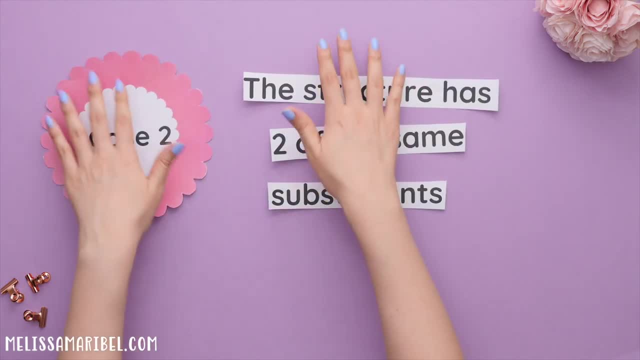 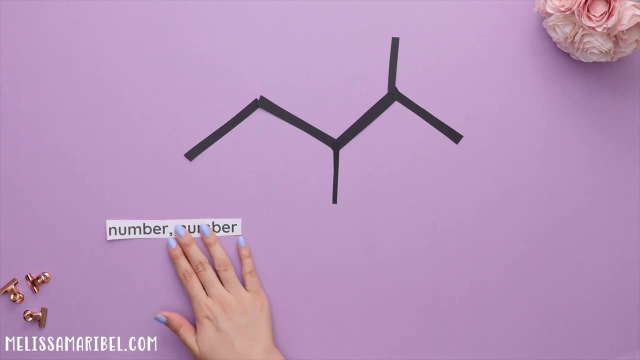 the structure has two of the same substituents. Here's how we'll format the name. Whenever a structure has two or more of the same substituent, we separate the numbers with a comma, then there's a dash. a prefix goes in front of the name of the substituent. 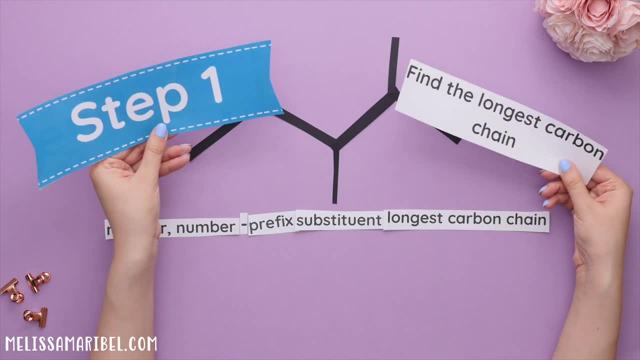 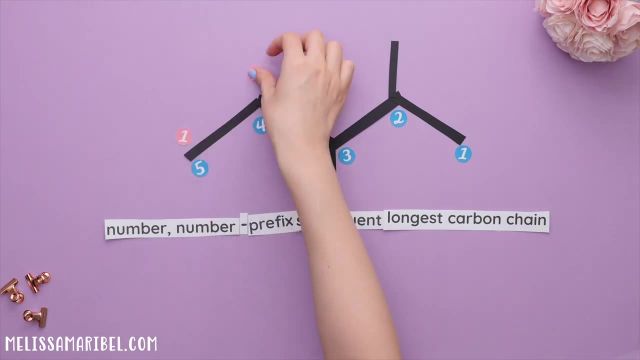 followed by the longest carbon chain. Step one: find the longest carbon chain. We have one, two, three, four, five this way, or one, two, three, four, five this other way. We know that 5 is the longest carbon chain. the prefix for 5 is pent, so pentane. 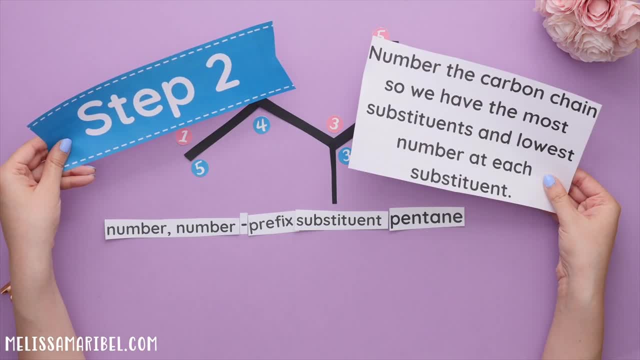 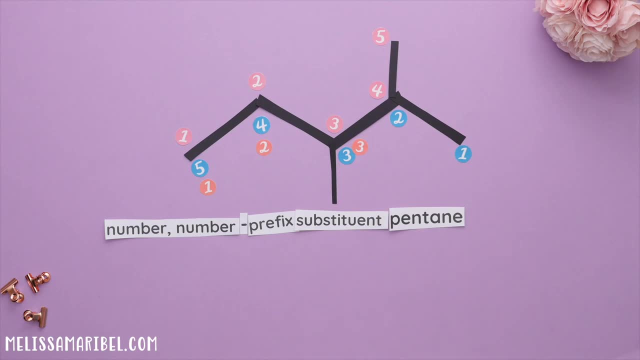 Step 2. Number the carbon chain. so we have the most substituents and the lowest number at each substituent. Here are some different ways we could have numbered this structure. This first one shows the substituents at 2 and 3,. the second one shows the substituents at 3 and 4, and this third one. 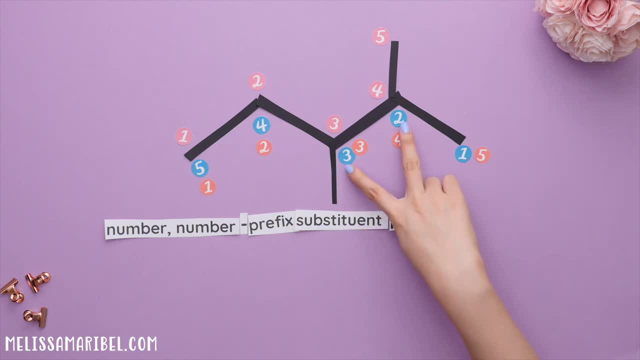 also is at 3 and 4.. The correct numbering is the first one, since we get the lowest possible number for substituents. so 2,3 goes in front. Step 3. Identify the types of substituents. We have two. 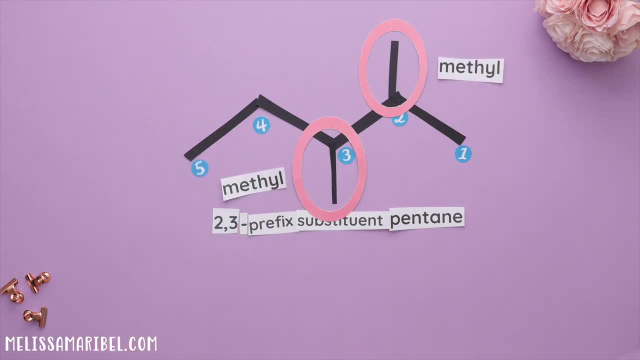 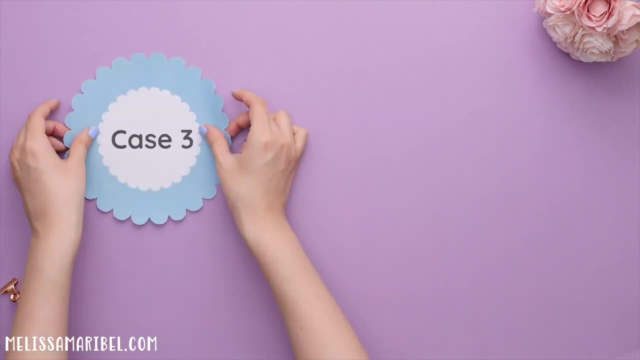 methyl groups. and since there are two of the same substituent, the prefix for 2 is di-, so di-methyl, and this is the name of our structure, Case 3.. The structure has two different substituents. Here's: how to identify the substituents. Here's how to identify the substituents. Here's how to identify. Here's how to identify the substituents. Here's how to identify the substituents. Here's how to identify them. Here's how to find the longest carbon chain Of the substituents that are present in the. 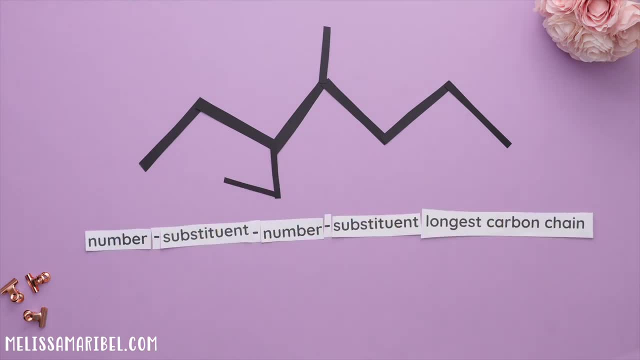 structure. we must remember which are the longest and longest, which means how long they are. Now figure out how we'll format the name With the two different substituent names and the number they are located at, followed by the longest carbon chain. Step 1. Find the longest carbon chain. We 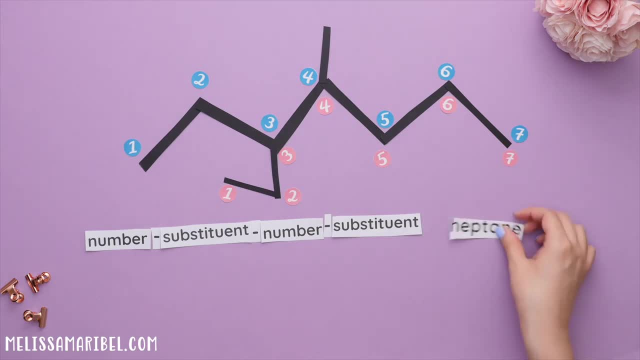 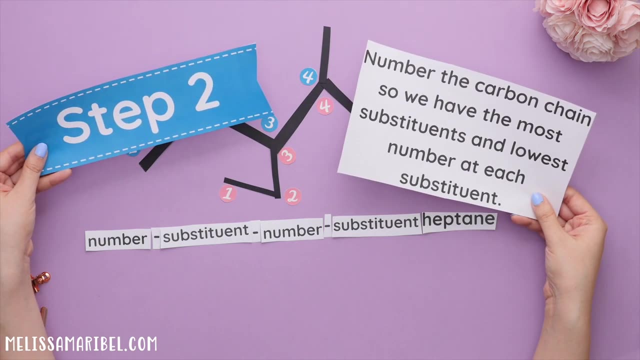 have 1,, 2,, 3,, 4,, 5,, 6,, 7,, or 1,, 2,, 3,, 4,, 5,, 6,, 7.. The longest carbon chain has seven carbons, so 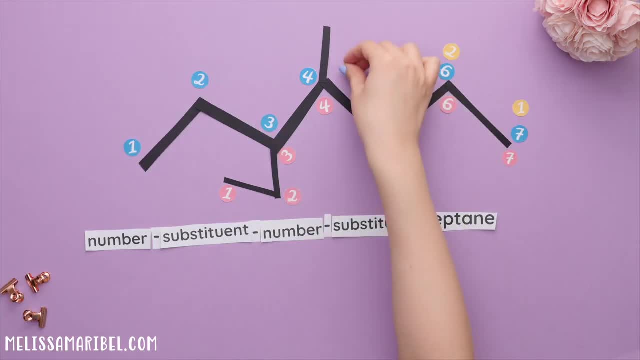 Here are some other possible ways we can number this. All the ways would give the same amount of substituents, but only ways 1 and 2 have the lowest number at each substituent. Way 1 and 2 will give you the same answer. I'll pick way 1.. 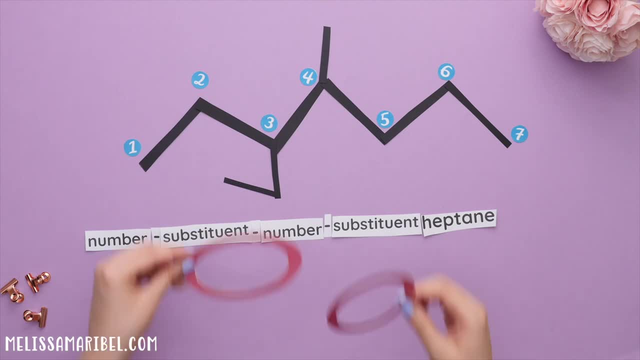 Step 3. Identify the types of substituents. We have a methyl and ethyl group. always write substituents in alphabetical order, So the ethyl goes first, then the methyl, and we'll place the numbers where each substituent is at. 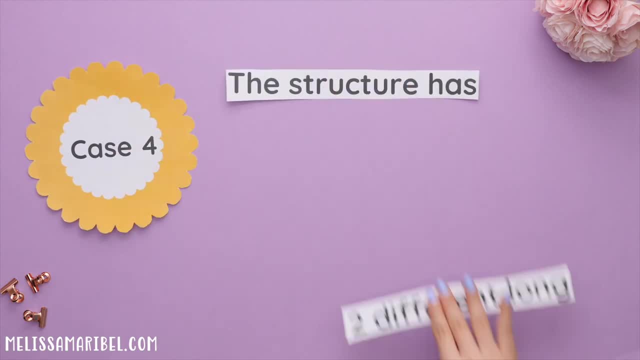 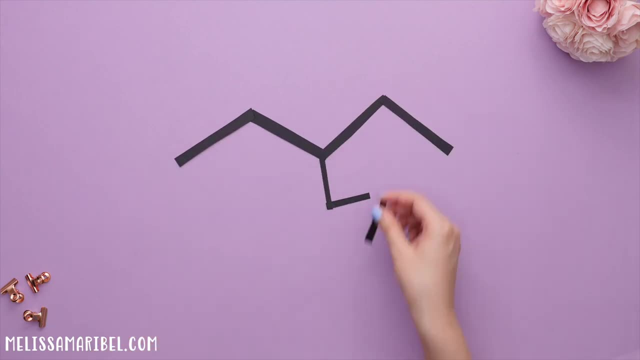 and this is the correct name: Case 4.. The structure has two different long carbon chains. Some structures have two completely different sized carbon chains, which we'll see here. So step 1. Find the longest carbon chain. Let's see what we have: 1,, 2,, 3,. 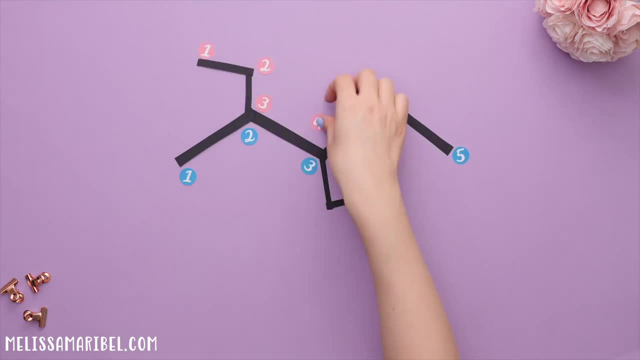 4,, 5, or 1,, 2,, 3,, 4,, 5,, 6, or 1,, 2,, 3,, 4,, 5,, 6, and 1,, 2,, 3,, 4,, 5,, 6, 7.. 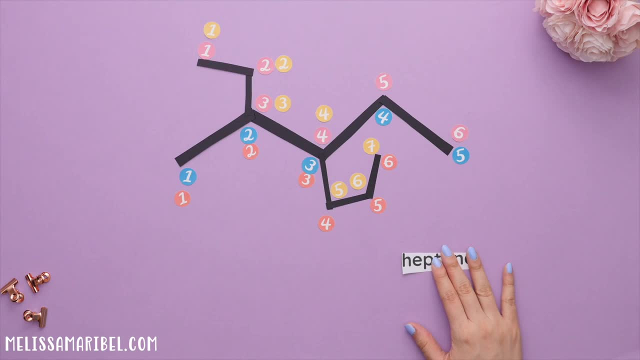 7 is the longest carbon chain, which is heptane Step 2.. Number the carbon chains so we have the most substituents and lowest number at each substituent. Here are two ways we could have numbered the chains. This first way is the best, since substituents are at 3 and 4.. 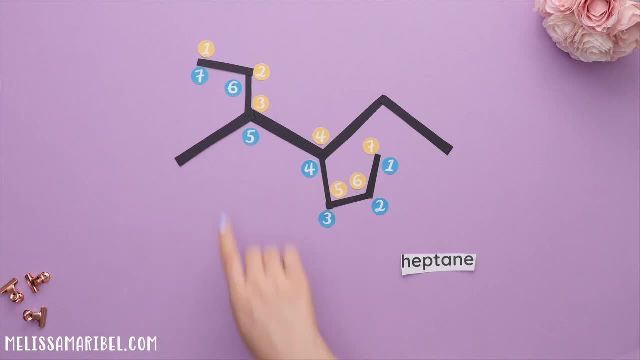 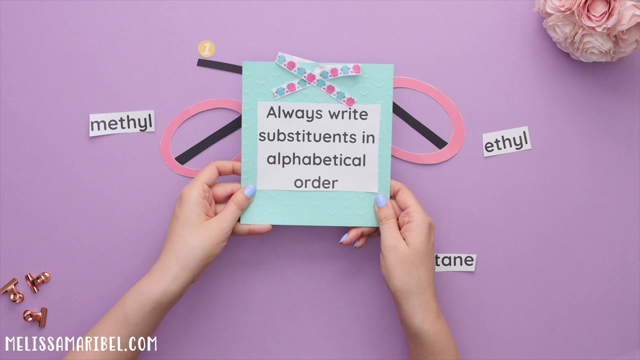 Rather than 4 and 5, because we always want the lowest numbers for each substituent. Step 3. Identify the types of substituents. We have a methyl group at 3 and an ethyl group at 4, and we always arrange our substituents in alphabetical order. When we do that, we get this: